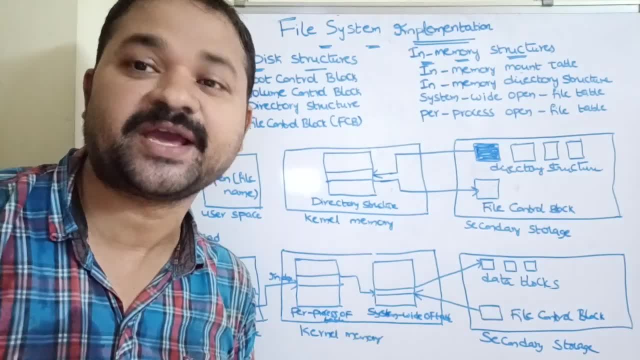 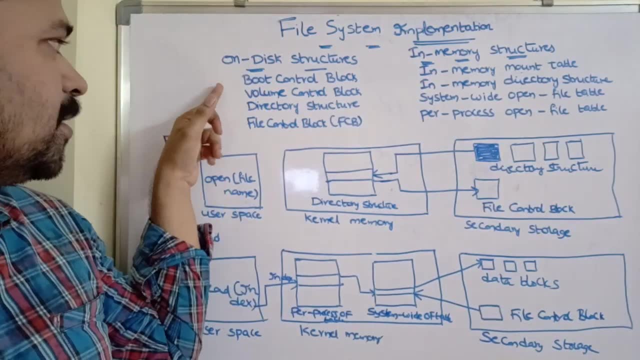 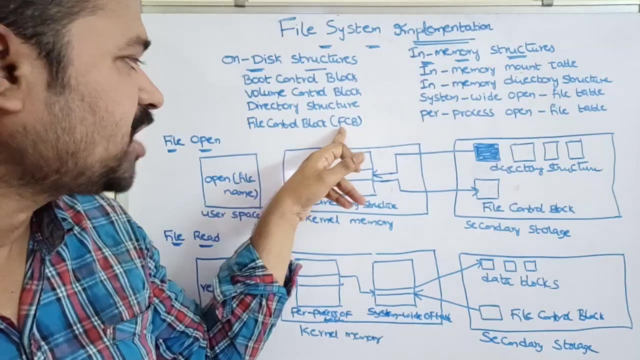 So that is nothing but kernel memory only. So kernel means important part of the operating system which resides in main memory. So let's see what are the on disk structures: Boot control block, volume control block, directory structure, file control block. In short, we can call as FCV. 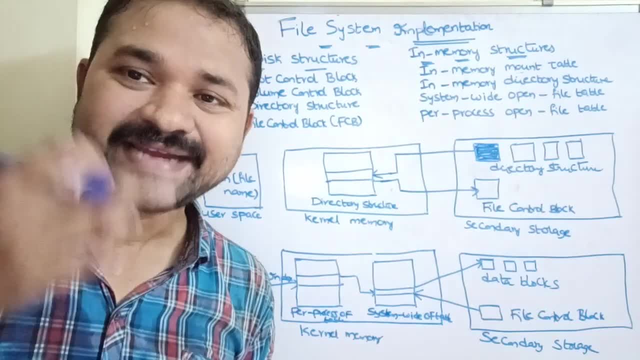 Let's see about the first one: Boot control block. It contains the information that is needed to boot an operating system. Generally, the hot disk is divided into two parts. The first one is on disk structure, The second one is on memory structure. So that is nothing but kernel memory only. So kernel means important part of the operating system which resides in main memory. 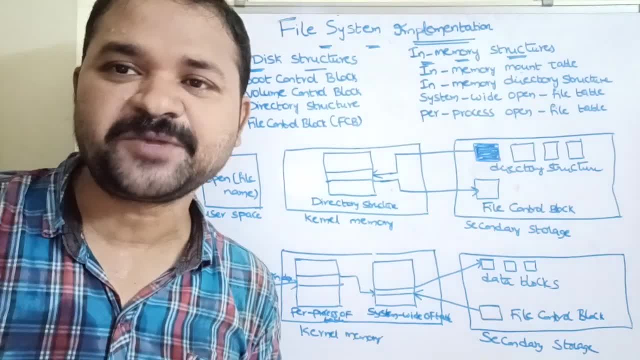 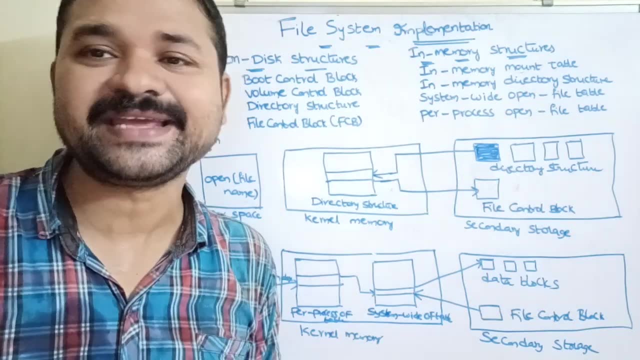 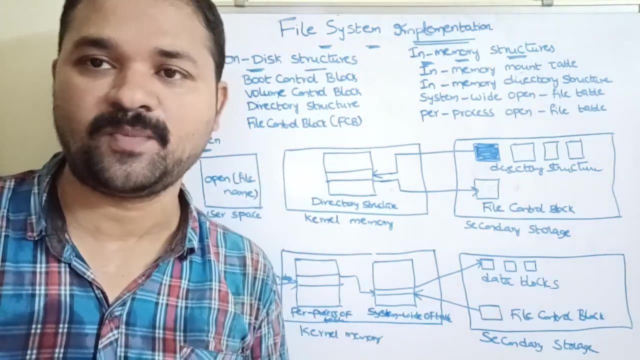 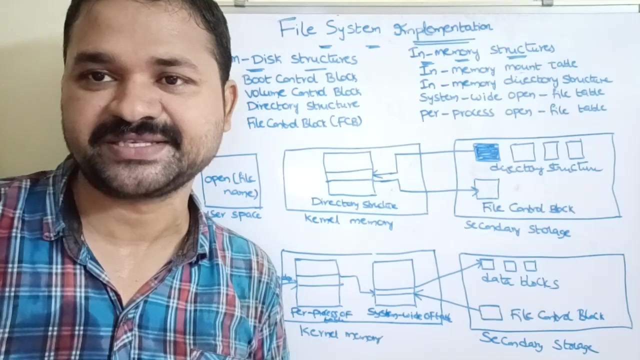 So the first partition is divided into several partitions, several volumes. The first partition is known as boot control block. The first partition contains the code that is needed in order to boot the operating system. So that is nothing but boot control block. And the second one is volume control block. It contains the information about that volume, that partition. We can have several partitions in the hot disk, So for each partition we can have a separate volume control block or partition. 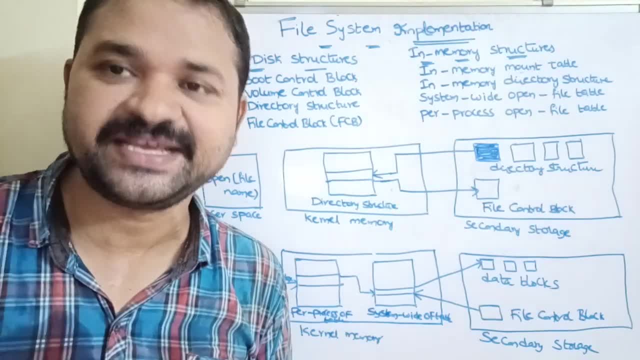 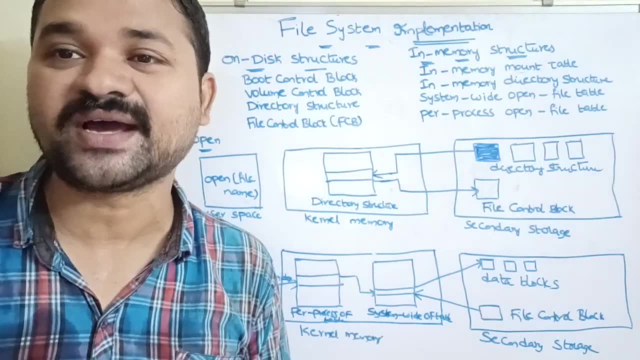 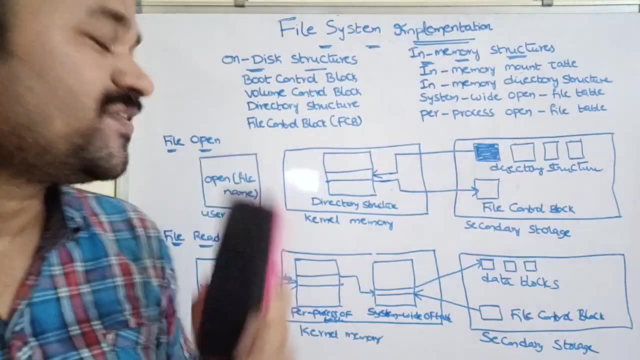 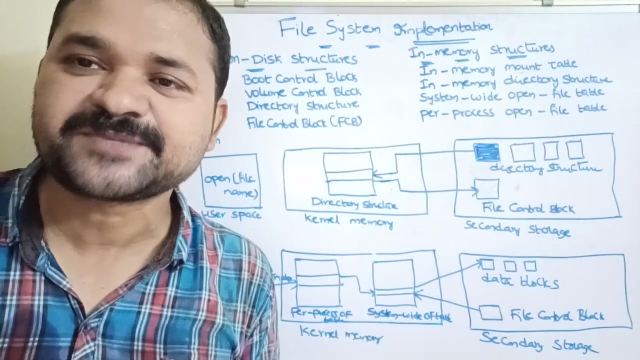 partition control block. The volume control block specifies information about how many blocks are there and what is the size of each block and how many free blocks are there. that everything that every block information will be available in volume control block. And the next one is directory structure. Directory structure is mainly useful in order to organize the files, So the corresponding files, the list of files, are present in the directory structure. 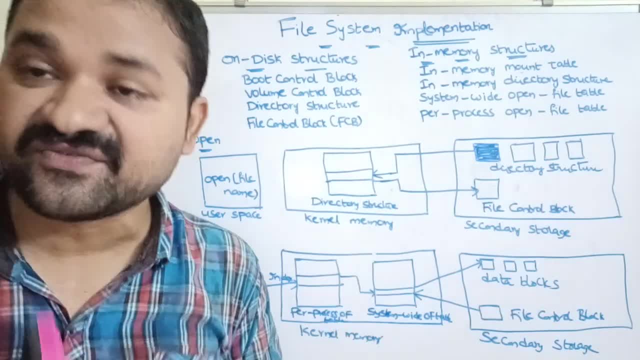 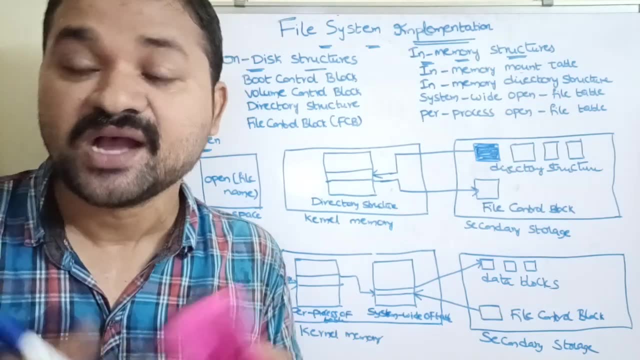 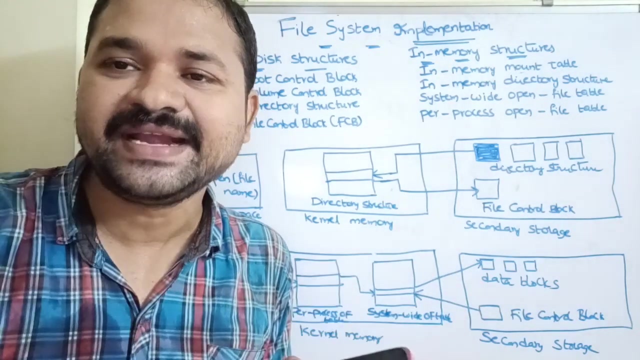 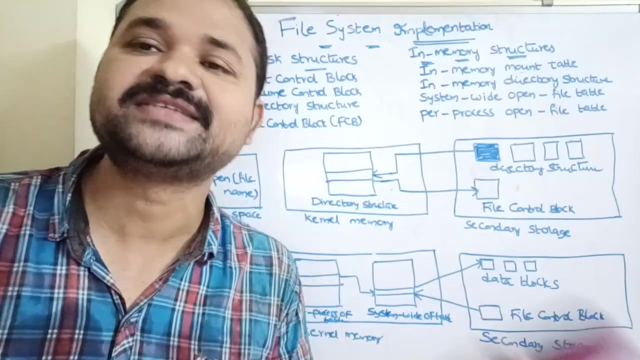 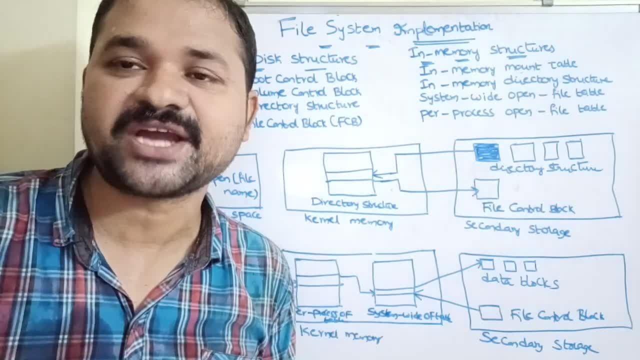 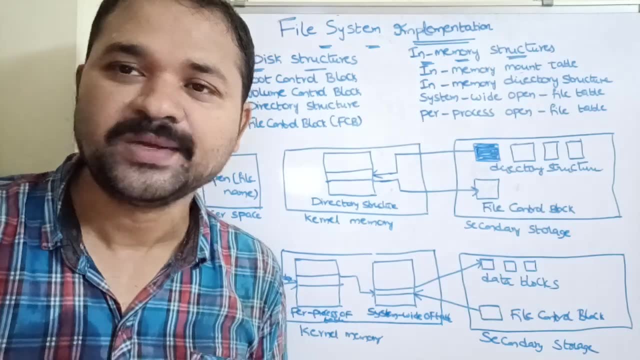 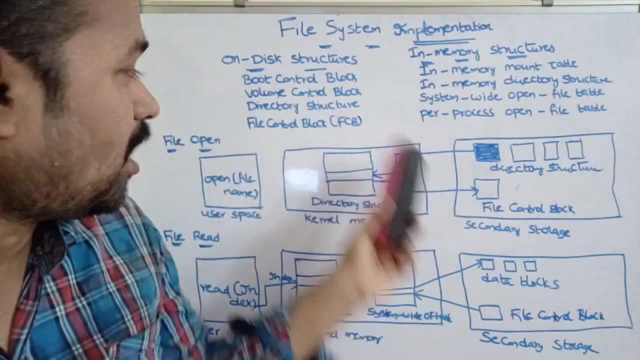 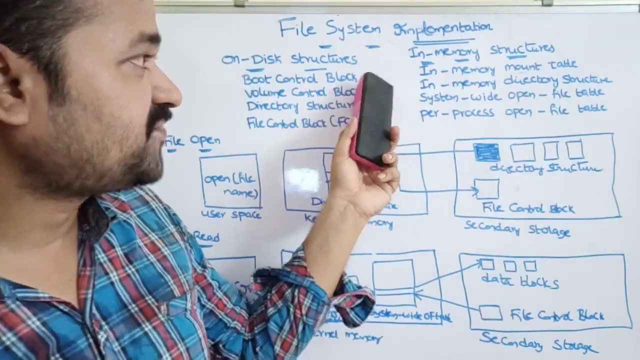 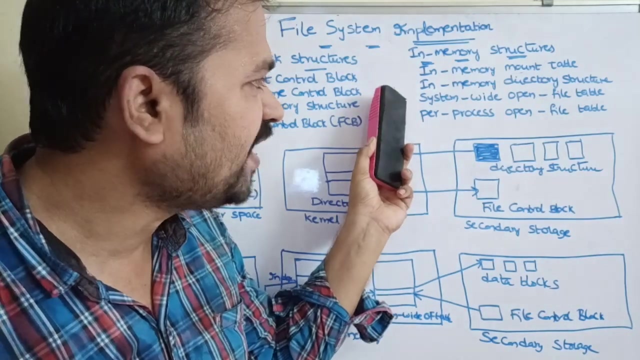 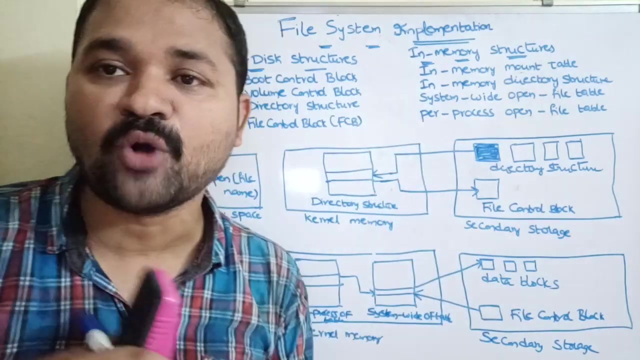 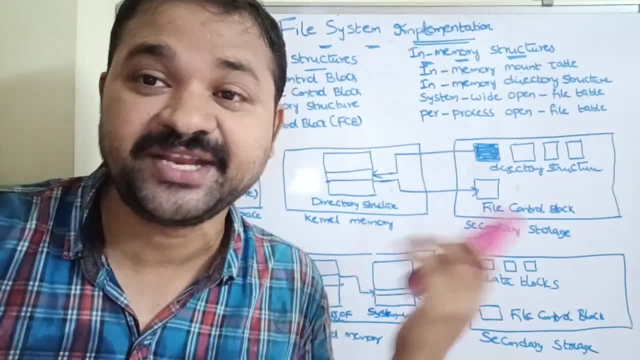 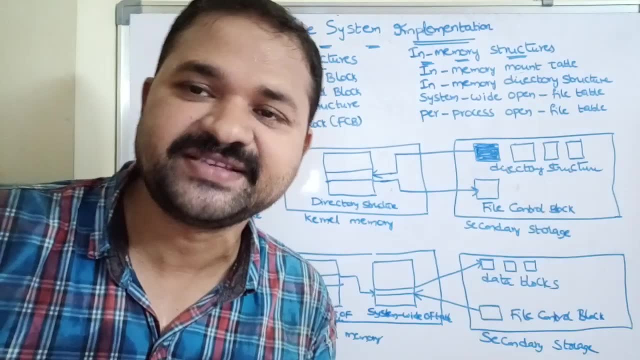 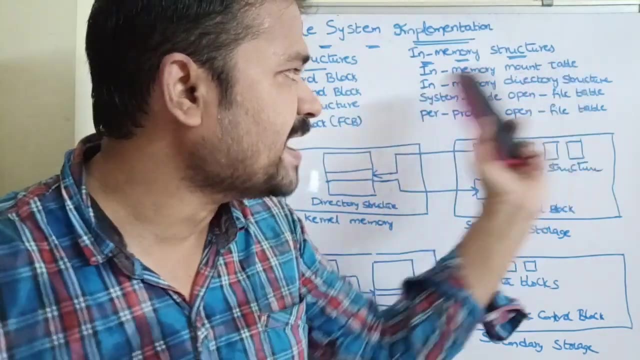 mount point at which location the corresponding directory structure is attached. so if there is a mounting, mounting means attaching files or directory structure to the one file system. one directory structure, okay, so that mounting information will be provided here and the next one is in-memory directory structure. here, this directory structure contains information about: 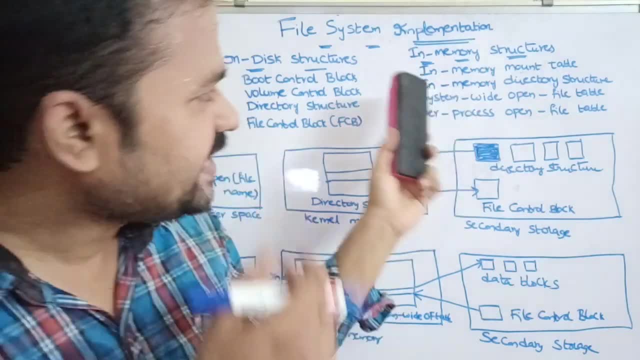 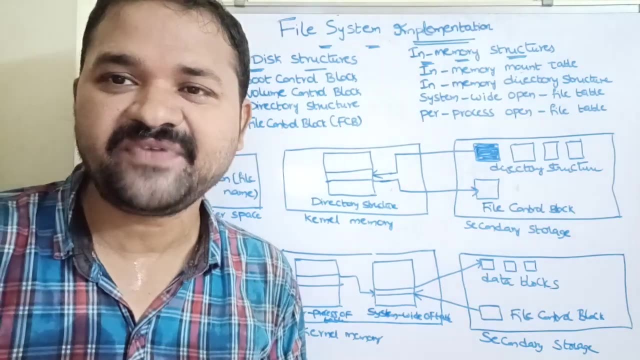 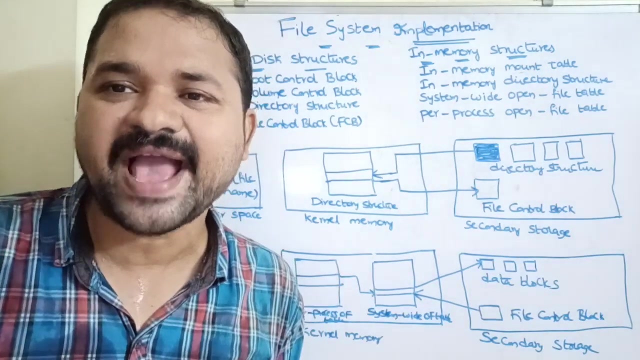 all the files which are present in the hard disk, whereas this in-memory directory structure contains the directories which are accessible recently. so let we have 100 hot. let we have 100 directories in the secondary storage. so, out of 100 directories, let we access five directories recently, so that information will be placed in in-memory directory structure. 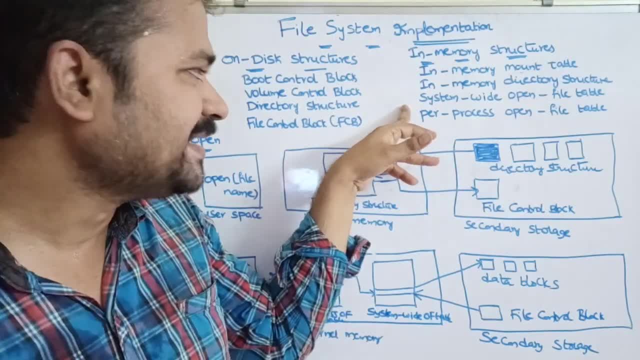 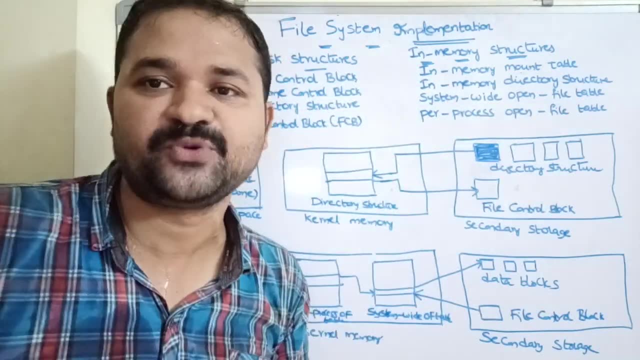 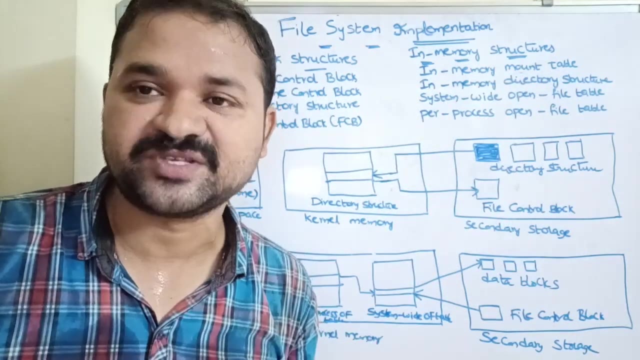 and next one is system wide open file table. the name itself specifies the meaning, so system means this file cable is belonging to the entire computer, so it contains the files that are opened by several processes. let we have 10 processes, so 10 processes opened. let us assume that 10 files. 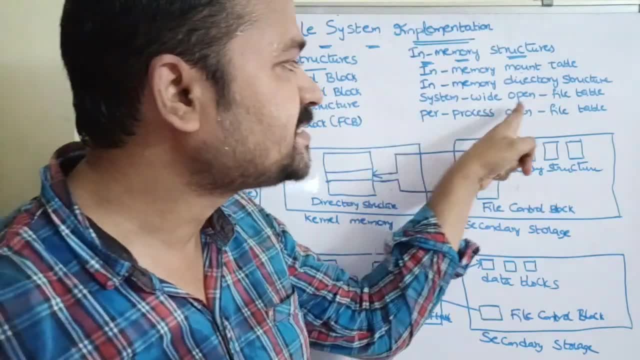 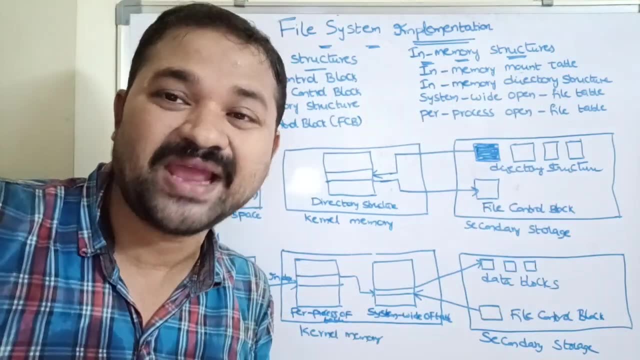 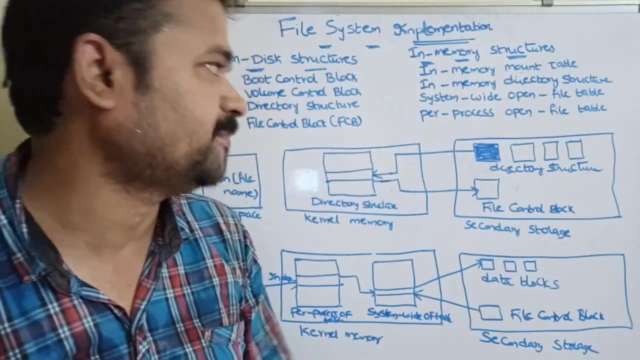 so those 10 files, information will be available in system by open file table. so it contains fcbs. a fcb means for each file. we can help file control block. so it contains the files which are opened by several processes in the system and the last one is per process open. 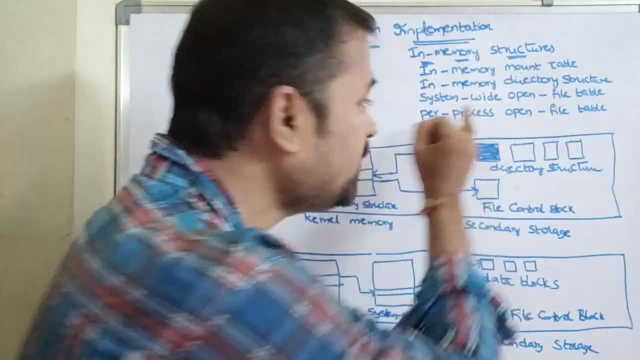 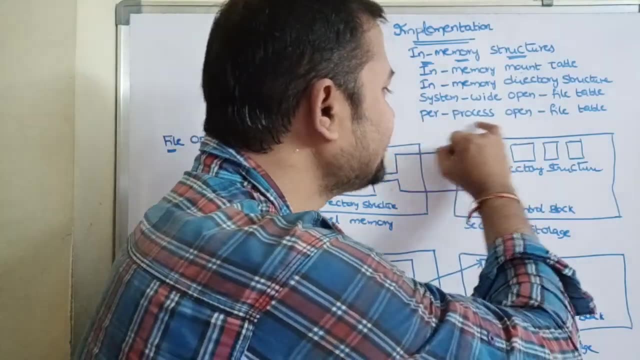 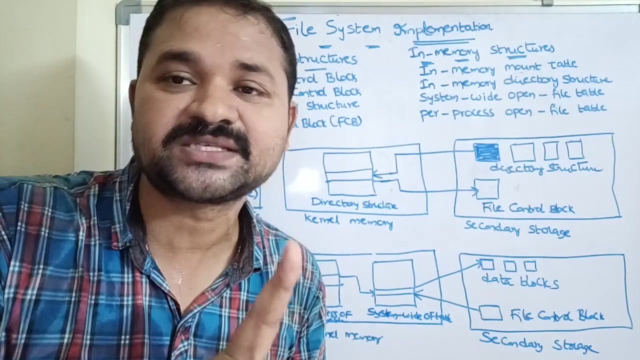 file table it contains the information about a single process. let us assume that a process open only one file so that file control block information will be resides in our process. open file table, so per process. open file table means it contains only one process. file. open information: various system wide open file table means it contains 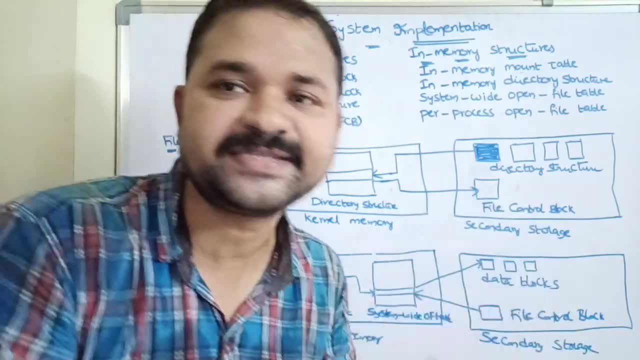 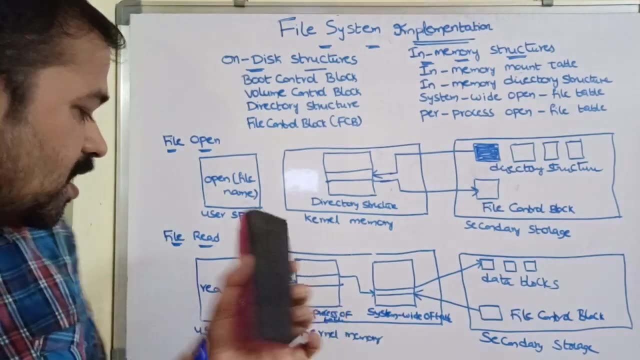 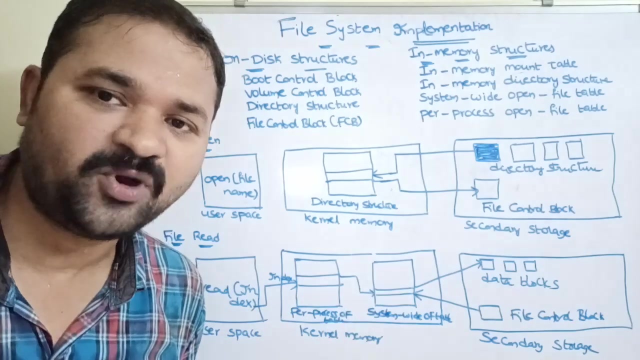 the information about all the files which are opened in the system. now let us take two function files. first one is open function call and the second one is read function call- how we can perform how internally read and open system calls are executed. so let's see with the help of these diagrams- the first one is 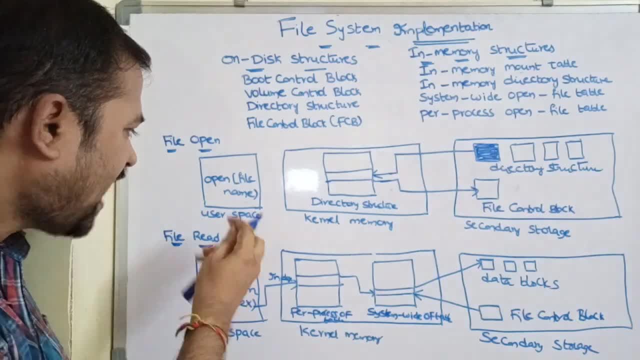 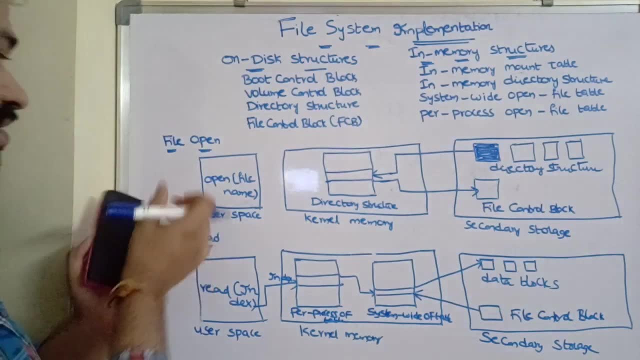 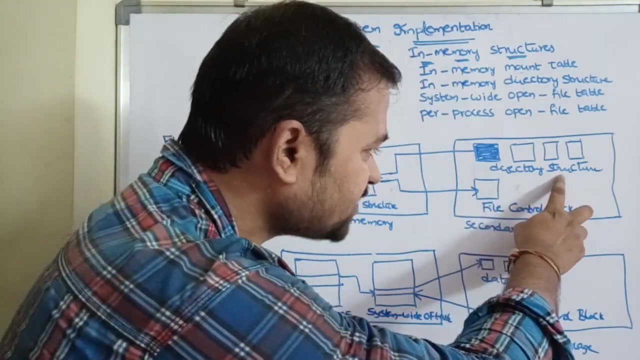 file open. so in order to open your file we have to specify file name as the input. so open file name as the input. so whenever we want to open a file, then first operating system pre-checks whether that file is presenting directory structure or not. this directory structure and file control block are 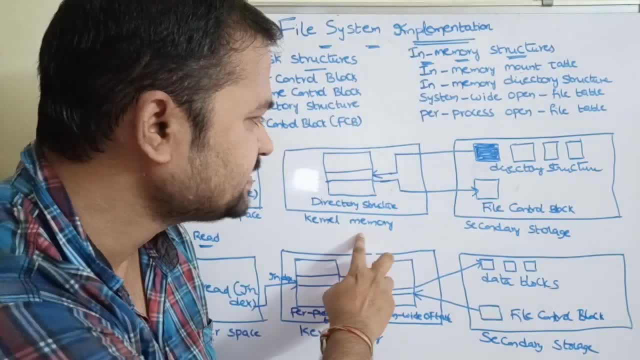 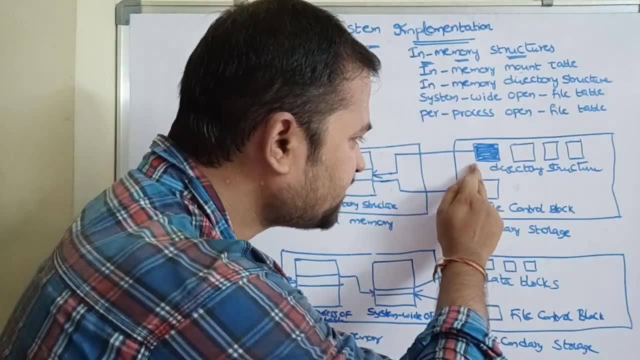 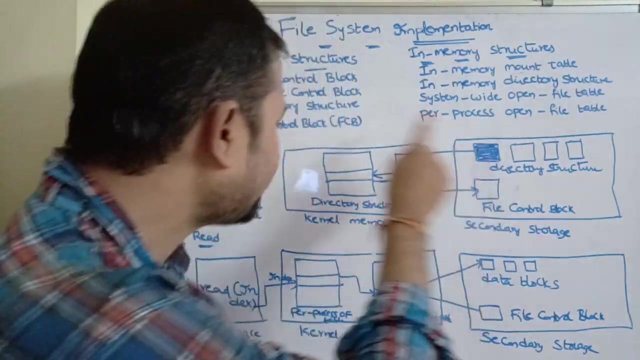 nothing but secondary storage. this is nothing but kernel memory. that is nothing but main memory. so whenever we given any file, then the operating system pre-checks whether that file is present in directory structure or not. let this is that file, so this file information will be transferred to the directory. 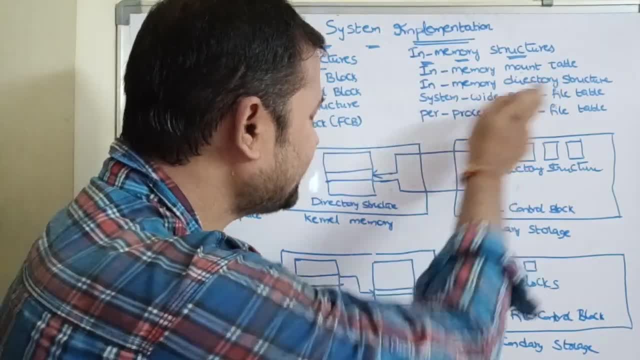 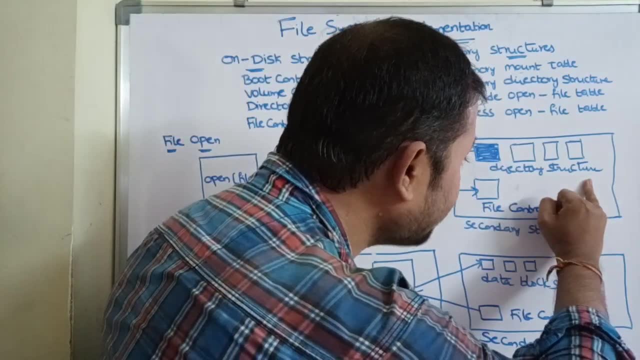 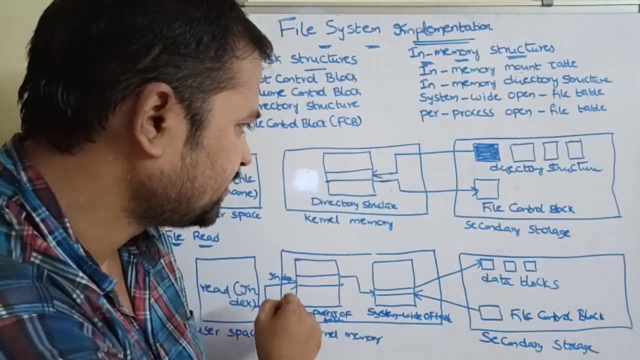 structure. so this directory structure is nothing but in memory directory structure. so for the next time, if you want to open that file, then instead of searching from secondary storage directory structure, directly operating system pre-checks in in this directory structure, in kernel memory directory structure, then after that. now we have a 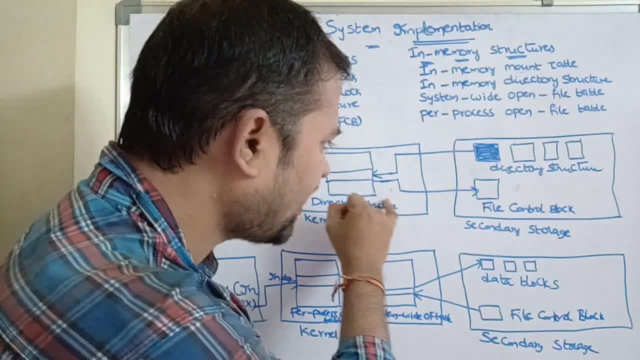 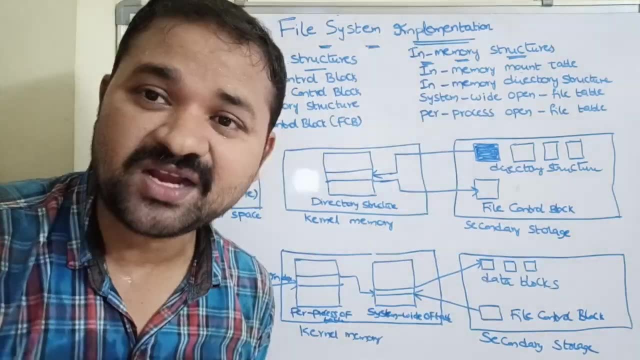 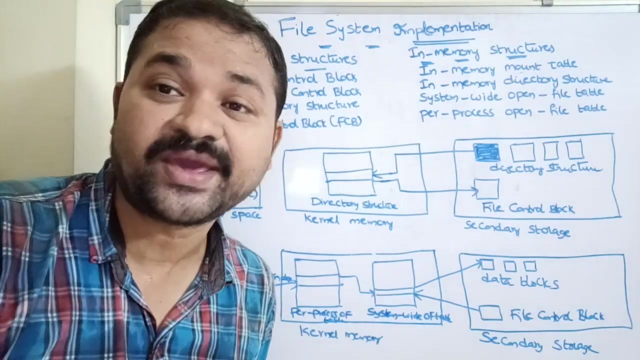 have that file information file name, so with the help of that file name operating system can access the file control block which resides in hard disk. so what is file control block? it provides the other information about that file, okay, such as what is the size of the file, what is the location. 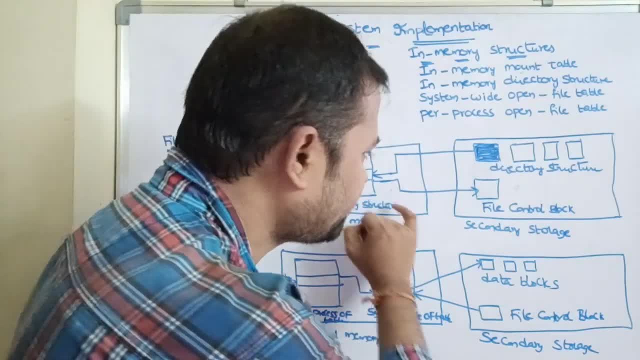 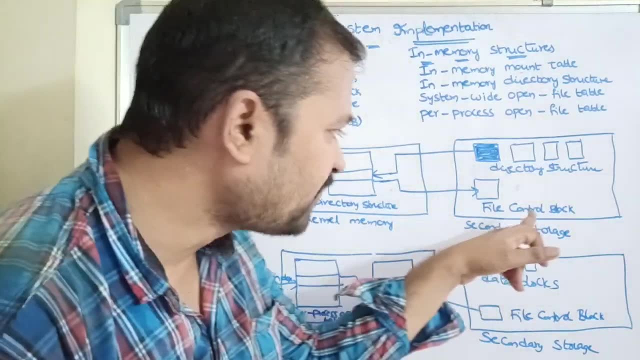 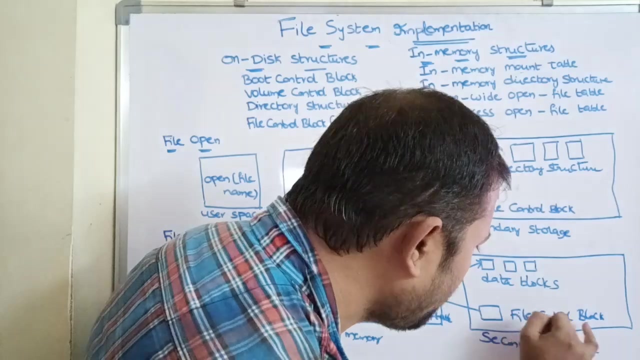 of that file. it can access all that information with the help of this file name, this file name entry. okay, so in this way, open function call is executed. here we have file control block, which provides information about that file. so next to what will happen is that file control. 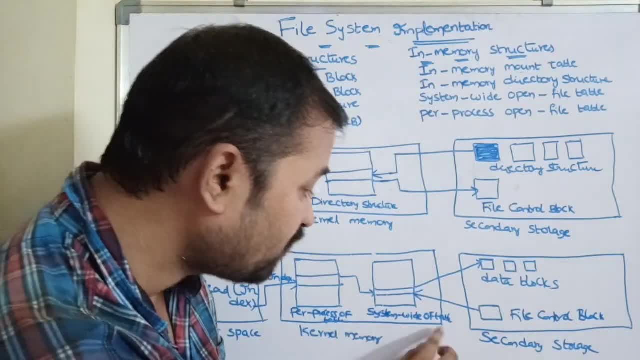 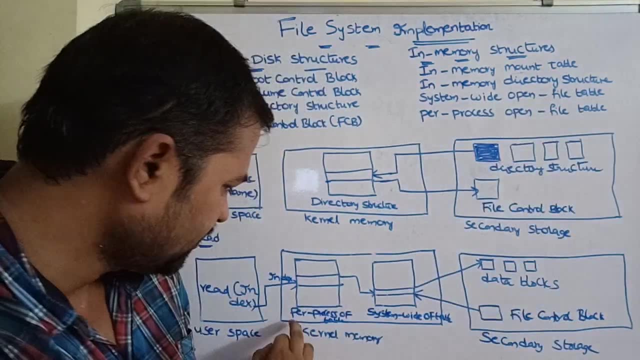 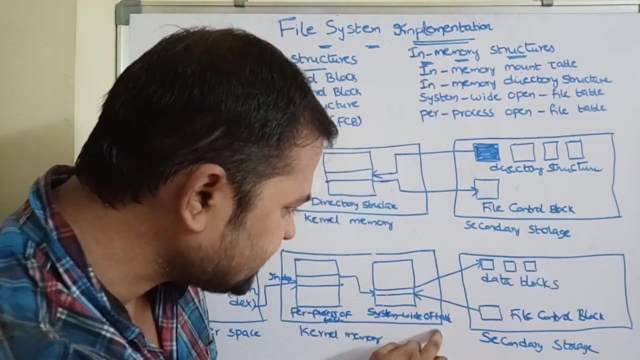 block information will be transferred to the system wide open file table for space constraints. here i am writing of of stands for system wide open file table. so this is nothing but part process open file table. here operating system transfers this file control block to the system wide open file table. why? because there is a possibility that we can access that file. 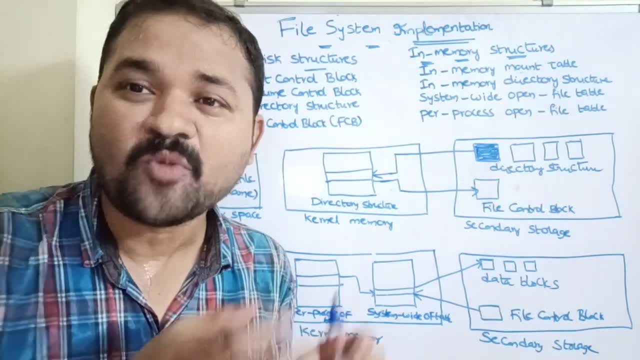 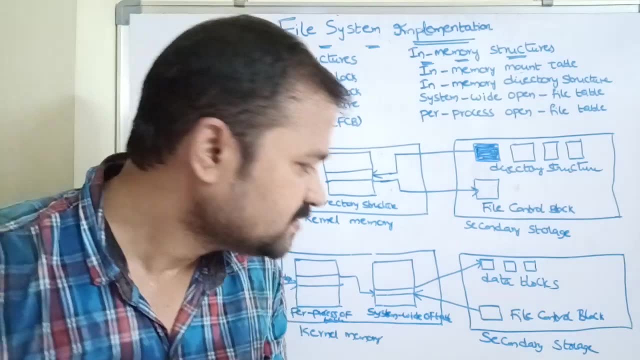 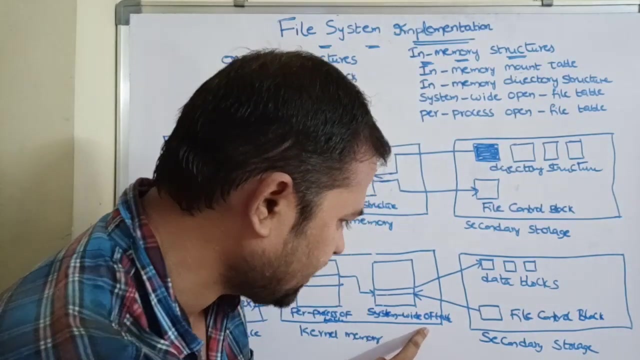 information several times. like we can perform operations on the file such as reading, writing, executing, we can perform several subsequent operations on that file. then, instead of retrieving from the secondary stories directly, operating system can access from the system wide open file table. why? because this is available in main memory so that cpu can access the data in a faster manner. 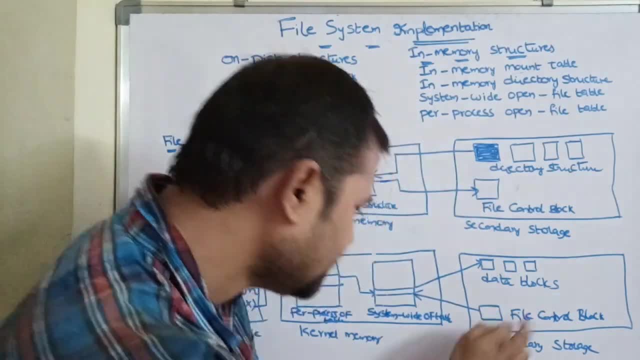 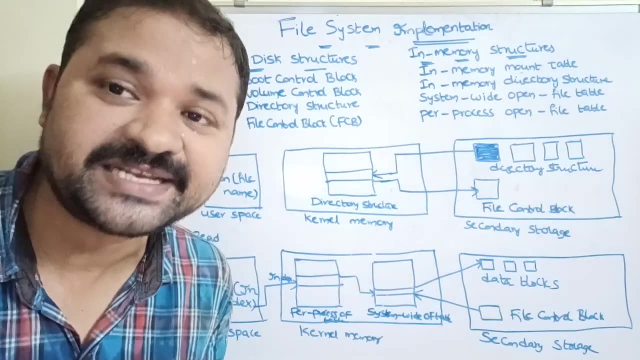 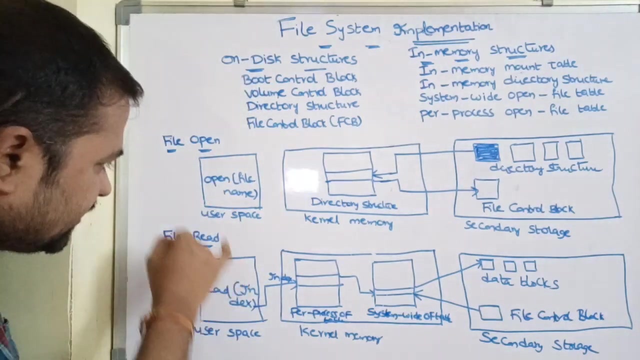 okay, so that's why this file control block information will be transferred to the system wide open file table. okay now, whenever a file is opened, whenever a file is created, then internally an identifier will be created, that file. so during read system call, what will happen is that file identifier is. that is nothing but an index, an integer value, that index, that. 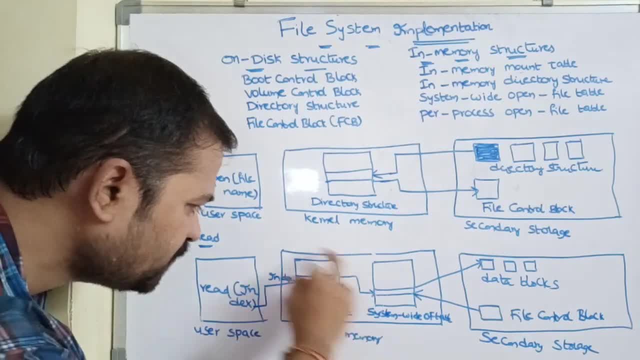 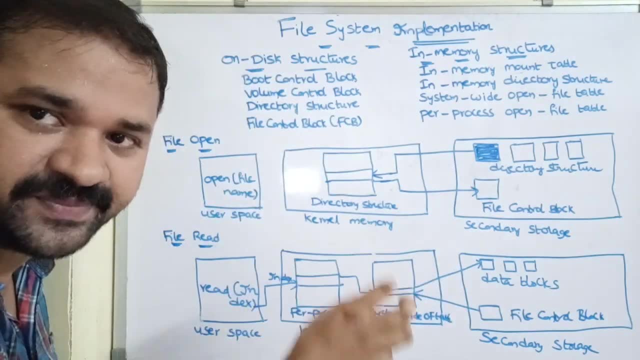 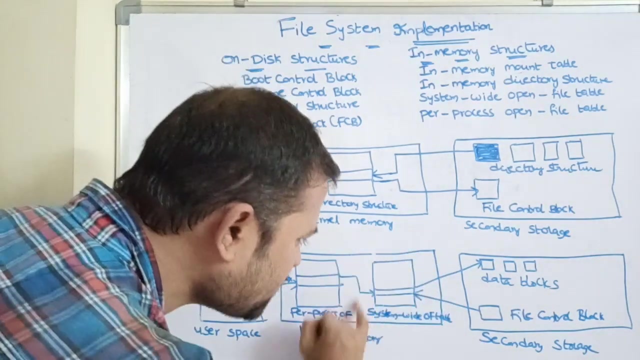 integer value. that file identifier will be given as input to the per process open file table. per process open file table contains the information about that file information. so it contains some fcbs file control block. that file control block points to an entry of the system wide open file table. why? because the system wide open file table contains several. 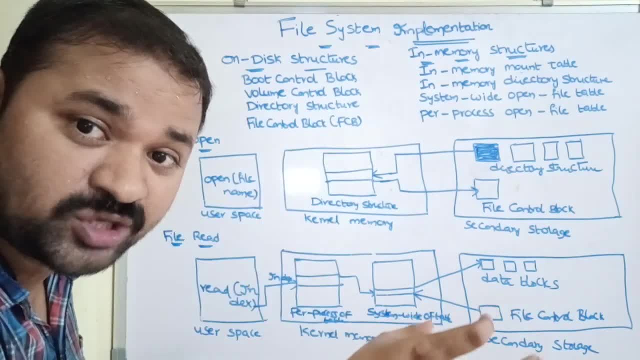 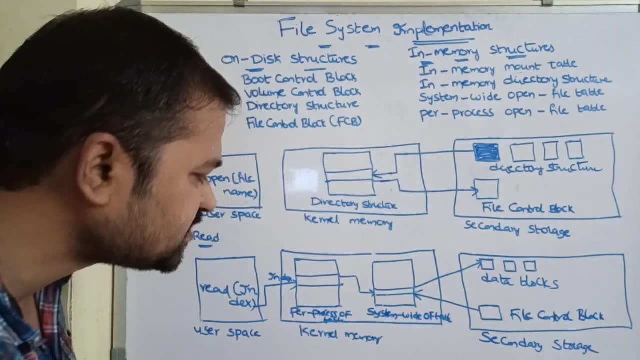 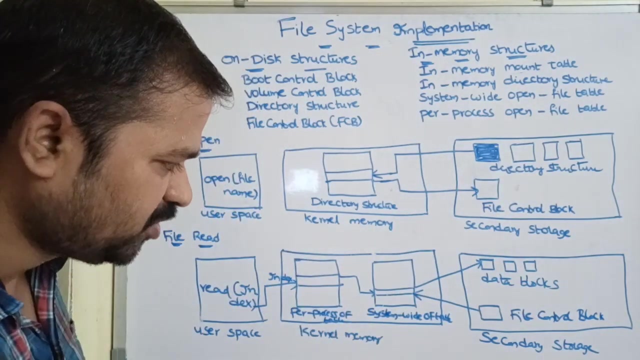 files, several files, fcbs. so out of all those files, so which file we, which file fcb we are accessing so that information is provided by the per process open file table, so it it contains fcb, that fcb will be given as input to the system wide open file table. so from 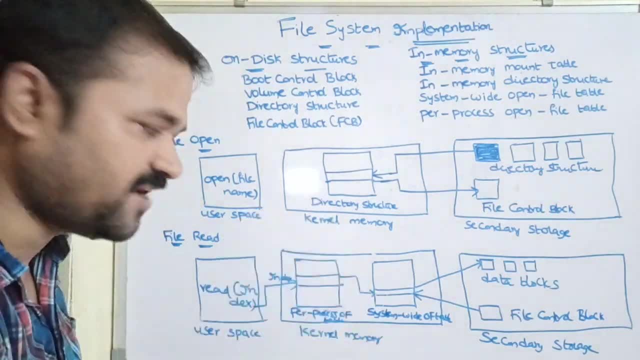 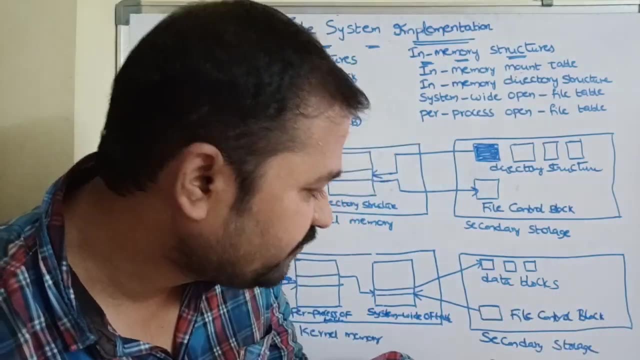 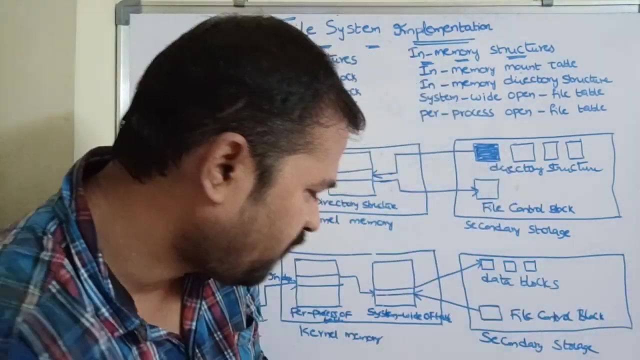 the system, wide open file table operating system will get fcb. so with the help of that fcb it can access the corresponding data blocks which are present in the secondary storage. this data block specifies the corresponding file is stored here, that we have five one, so that file, that file one is stored here in these three blocks. okay, so if you want,